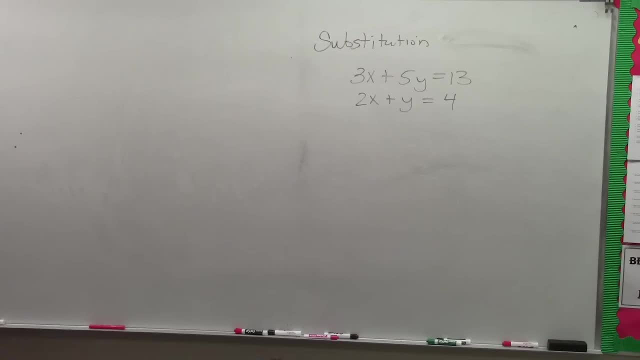 All right. So, ladies and gentlemen, what we have here is we are going to solve the system by substitution. Now, this we could solve by graphing, right? It's the same thing. But rather than getting out graph paper and trying to do all the graphing method, we can also use an algebraic method. okay. Now, the important thing is still: we're going to have our consistent, inconsistent solutions, dependent and independent, And I'll kind of talk about those. I'll kind of talk about what those different solutions mean algebraically. But in the substitution method, we want to use a. 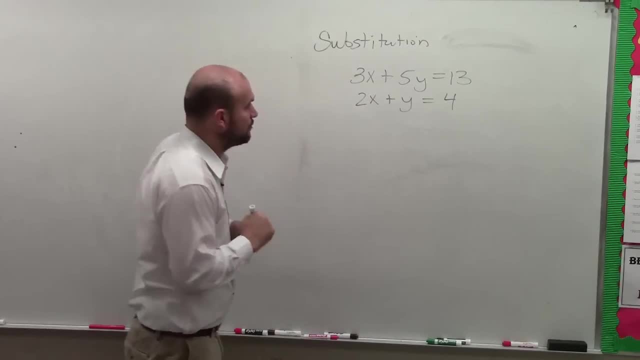 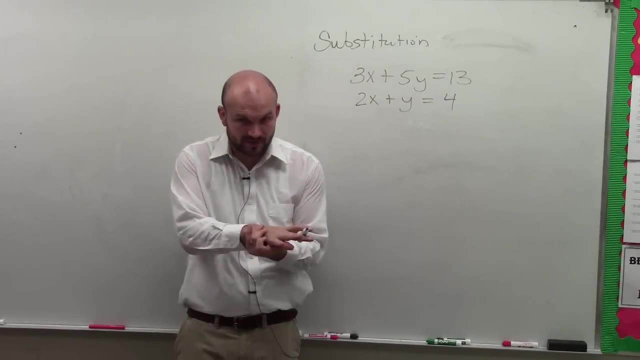 substitution method. The best time to use substitution is when you guys might want to write this down. I'm not going to write it down for time purposes, But whenever you have a variable that is solved, or meaning anytime you have a coefficient for one of your variables. 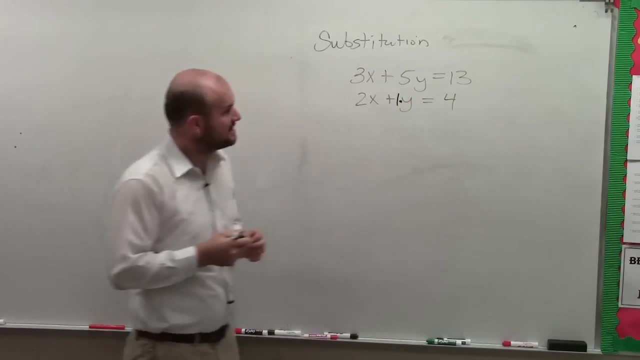 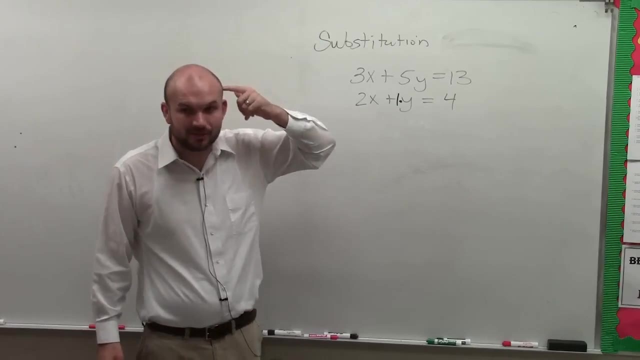 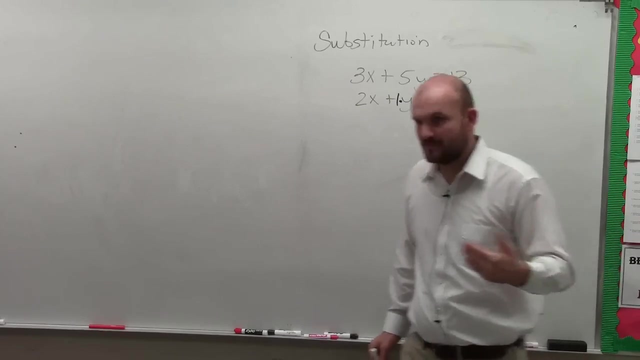 and that is either one or negative one. So you guys can see, right there, y has a coefficient of one, right? So mentally in my brain I'm going to want to use substitution. So anytime you have a variable that has a coefficient of one or negative one, Lizzie, it is going to be beneficial. 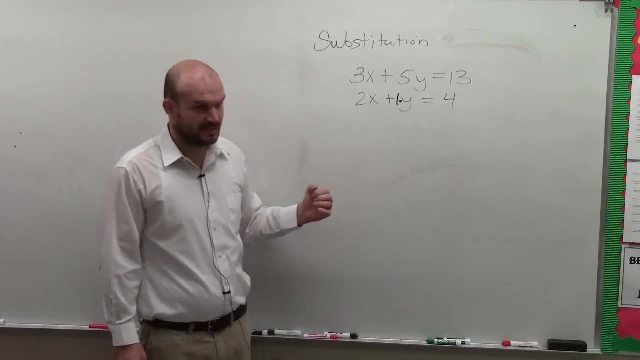 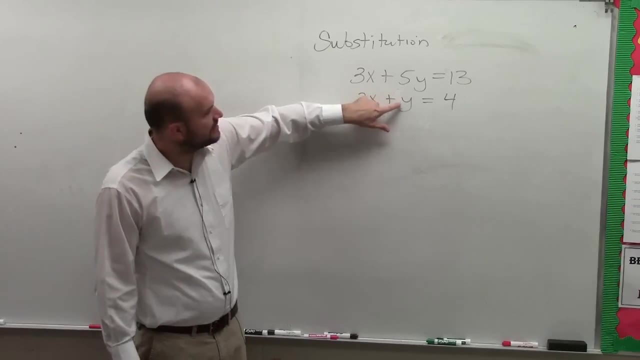 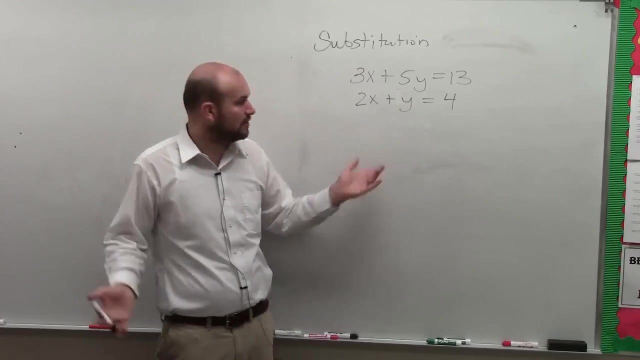 for you to use substitution Make sense. So how do we use substitution And why is it important when we have a coefficient of one? The reason being is because whatever variable has a coefficient of one or negative one, and even if you have two of them, just pick which one you want to solve for. 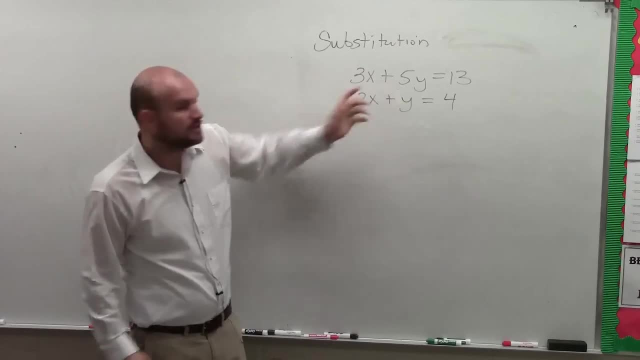 But this is the only variable that has a coefficient of one, correct? So what I'm going to do is I am going to solve for that, Because when it has a coefficient of one, I don't need to undo multiplication or division, right? 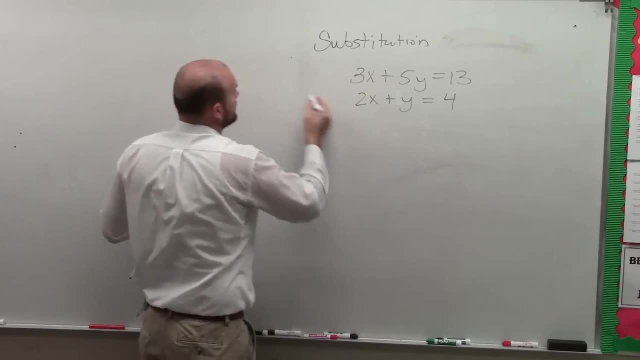 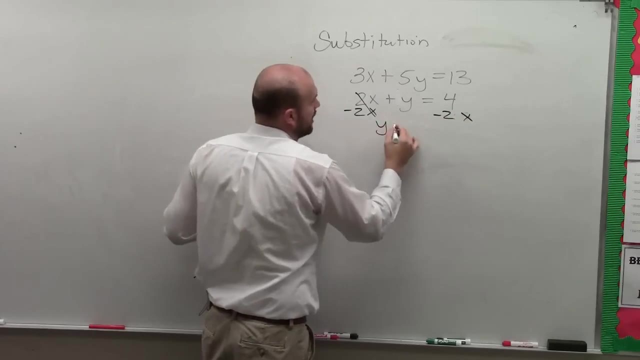 I just need to undo addition or subtraction. So I'm going to subtract a 2x from both sides. Therefore, now I have y equals negative 2x plus 4.. So now I'm just going to rewrite my system. 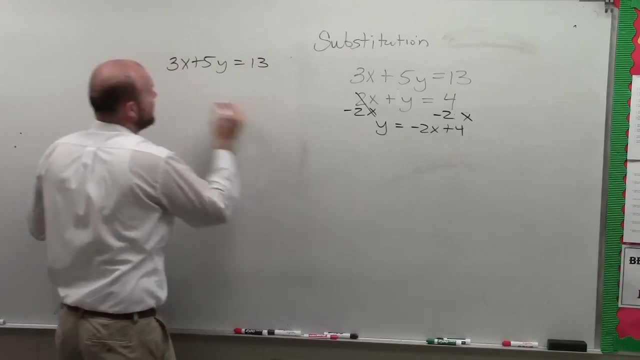 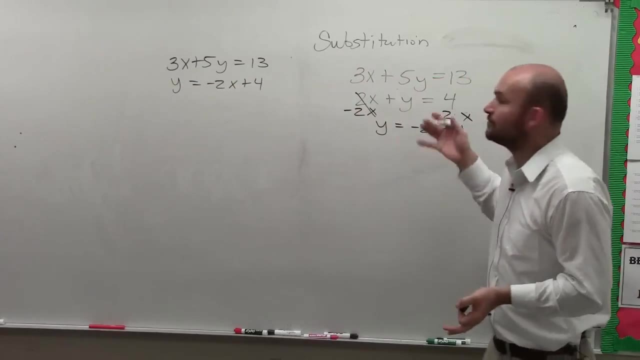 It's 3x plus 5y equals 13, and then y equals negative 2x plus 4.. So basically, when we're doing these functions, we're just going to be able to have it written with a variable isolated. 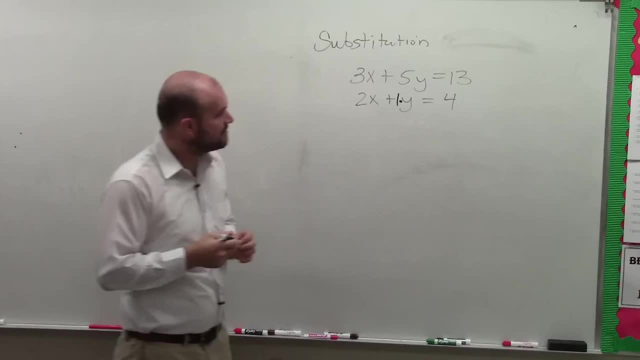 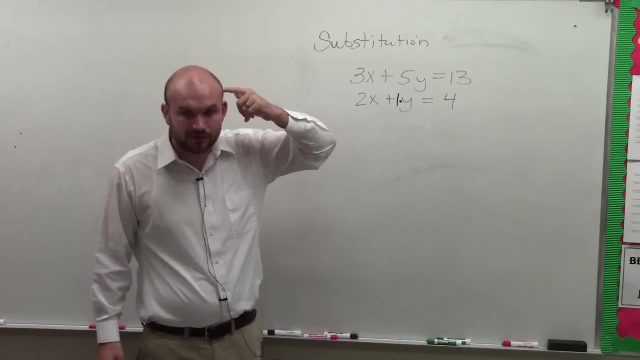 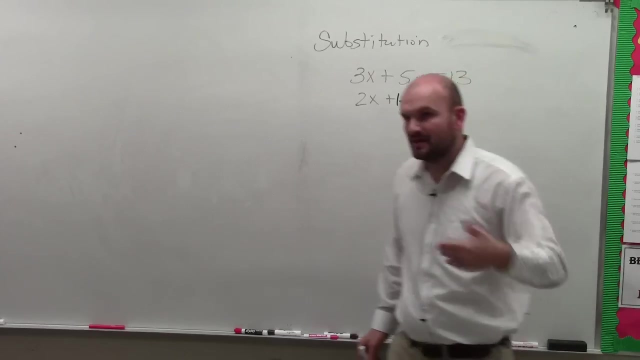 and that is either one or negative one. So you guys can see right there y has a coefficient of one, right? So mentally in my brain I'm going to want to use substitution. So anytime you have a variable that has a coefficient of one or negative one, Lizzie, it is going to be beneficial for you. 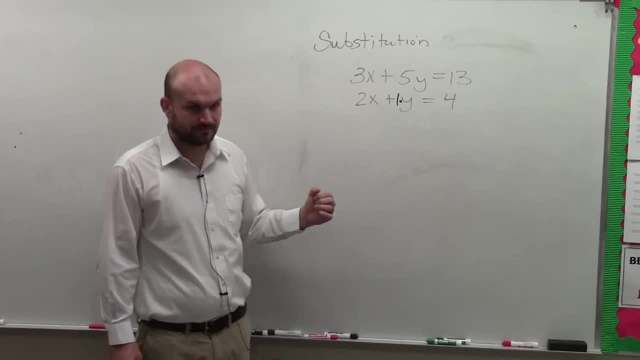 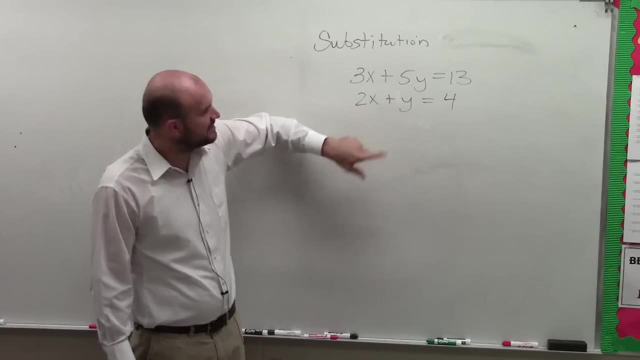 to use substitution Make sense. So how do we use substitution and why is it important when we have a coefficient of one? The reason being is because whatever variable has a coefficient of one or negative one, and even if you have two of them, just pick which one you want to solve for. But 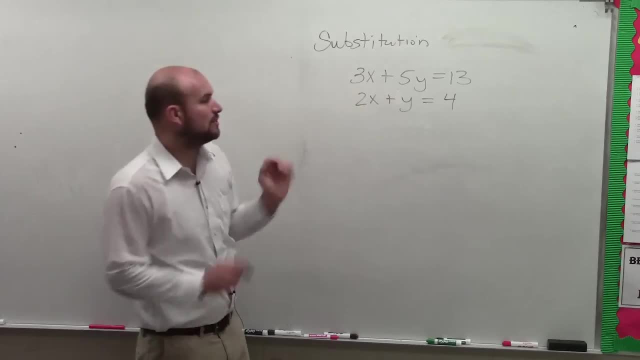 this is the only variable that has a coefficient of one, correct? So what I'm going to do is I am going to solve for that variable, Because when it has a coefficient of one, I don't need to undo multiplication or division, right, I just need to undo addition or subtraction. So I'm going to. 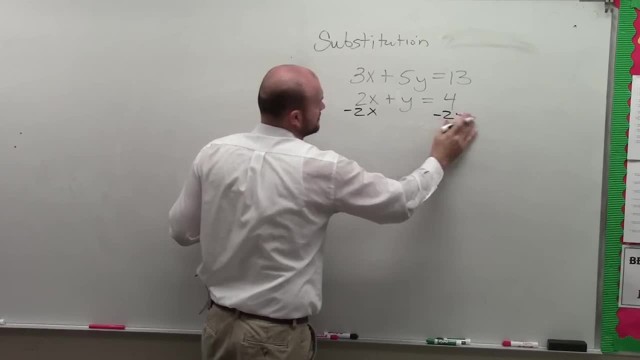 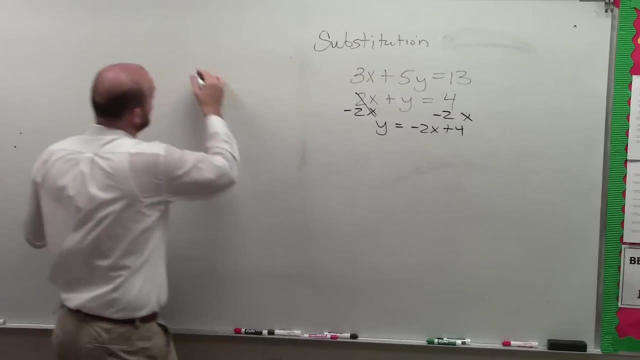 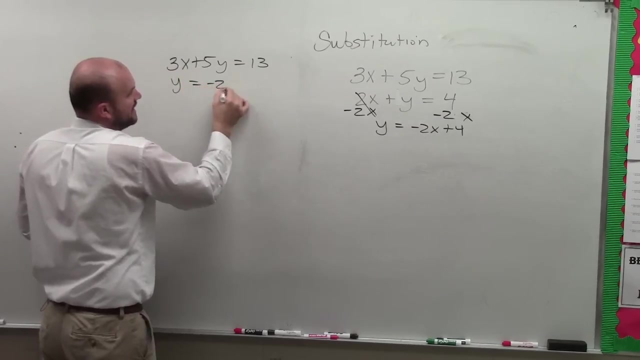 subtract a 2x from both sides. Therefore now I have y equals negative 2x plus 4.. So now I'm just going to rewrite my system. It's 3x plus 5y equals 13,, and then y equals negative 2x plus 4.. So 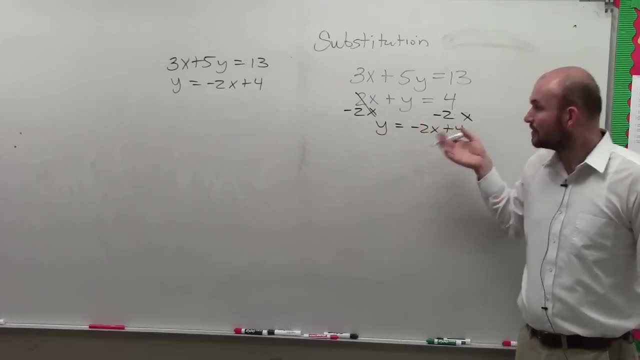 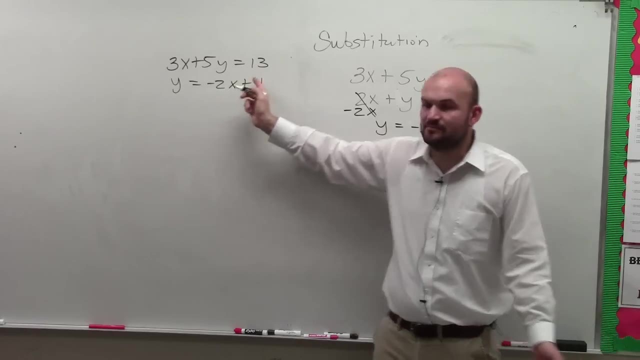 when we're doing substitution, we want to be able to have it written with a variable isolated. all right, And you can do this when it's not equal to one, but then you'd have to undo multiplication or division. So it's easiest when you have a variable that has a coefficient of one. 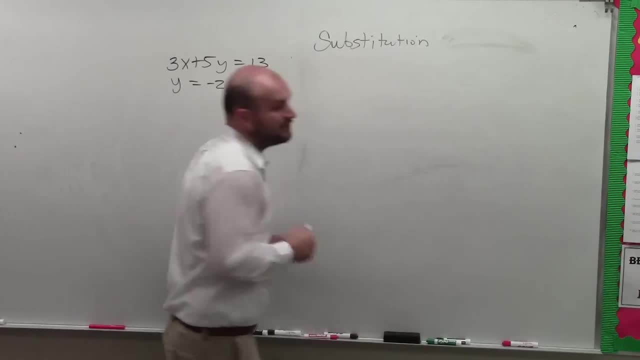 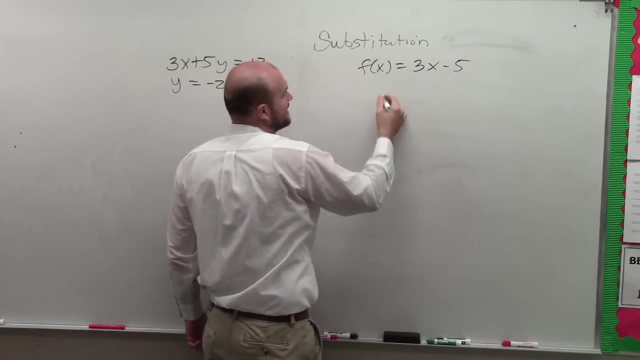 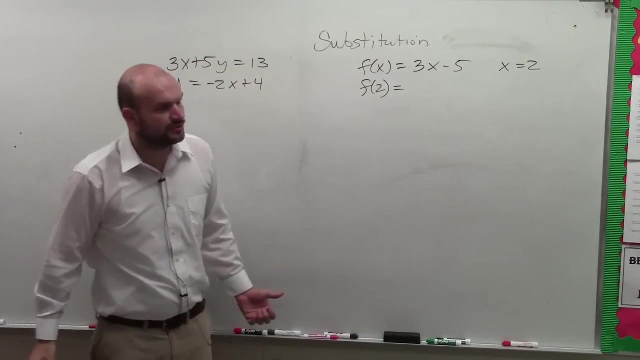 So now, if you guys remember when we did functions, if I had f of x equals 3x minus 5, and I say: find when x equals 2.. Or I said they would say f of 2.. Now, what else did we do with the 2?? You put it in for the x, right? 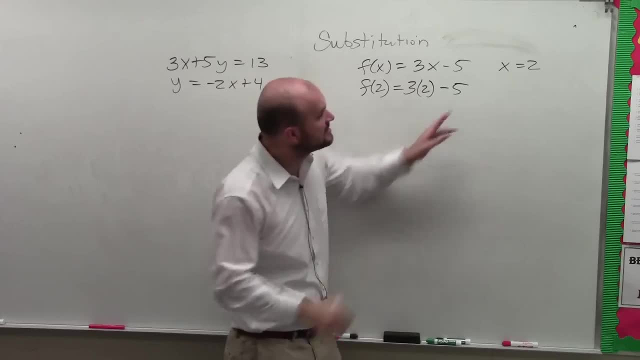 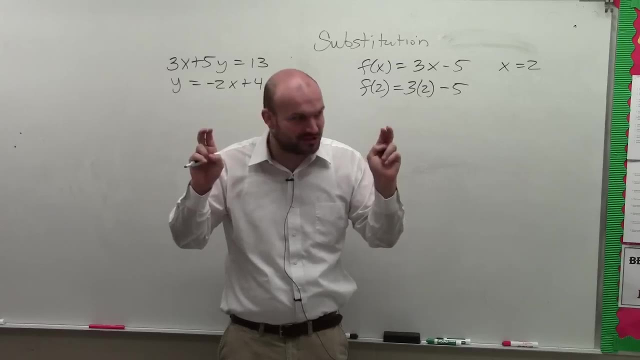 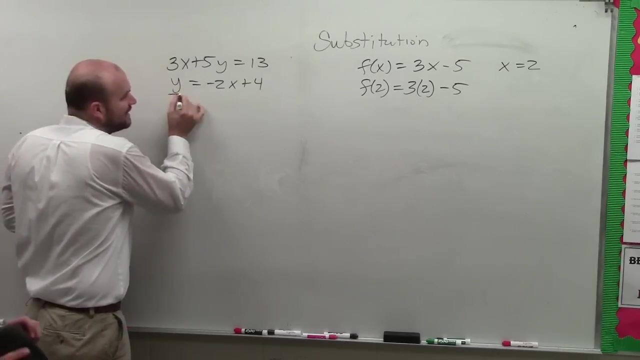 So you did 3 times 2 minus 5, because x was equal to 2.. 2 was equal to x. You could replace them or substitute one for the other, correct? Now we're doing something very, very similar. Now y is not. 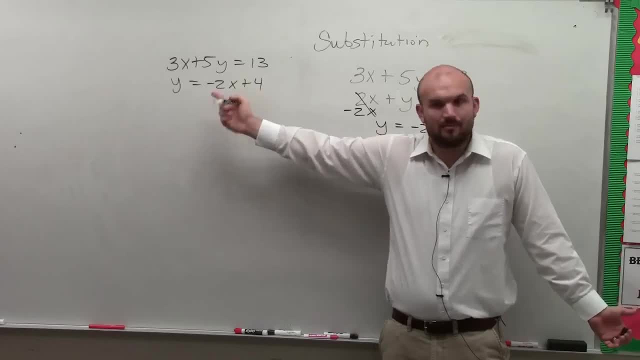 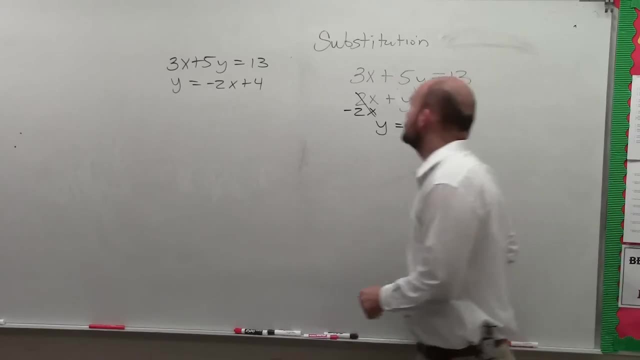 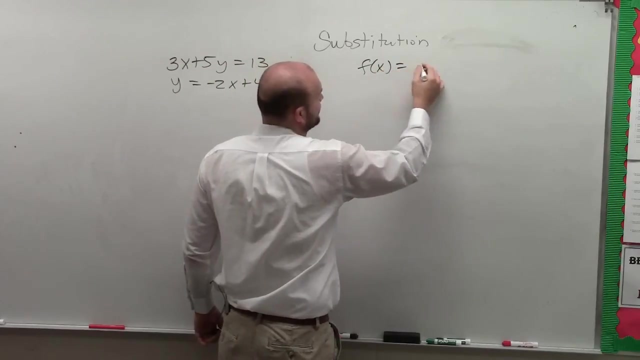 Alright. And you can do this when it's not equal to one, but then you'd have to undo multiplication and division. So it's easiest when you have a variable that has a coefficient of one. So now, if you guys remember when we did functions, if I had f of x equals 3x minus 5, and I say: 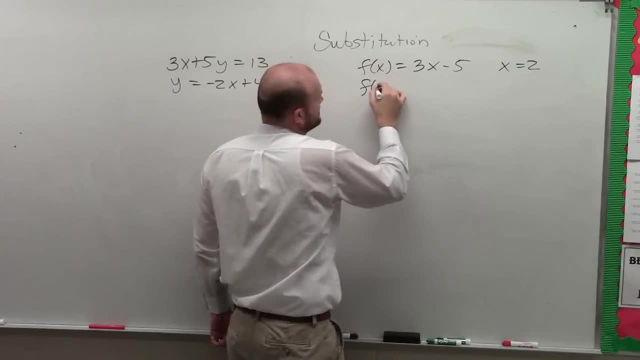 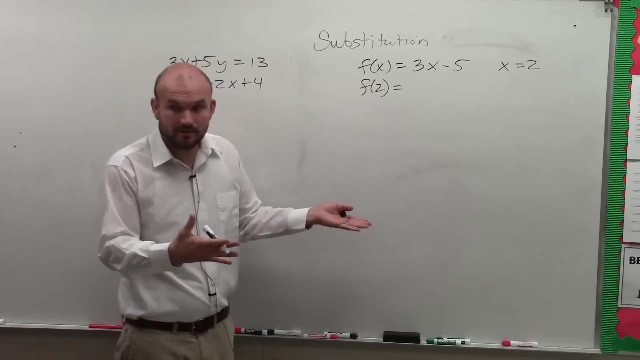 find when x equals 2.. Or I said they would say F of x equals 2y, and then y equals 2y, and then y equals 2y, And if I had, I would say of two. Now what else did we do with the two? You put it in for the x, right? So you did. 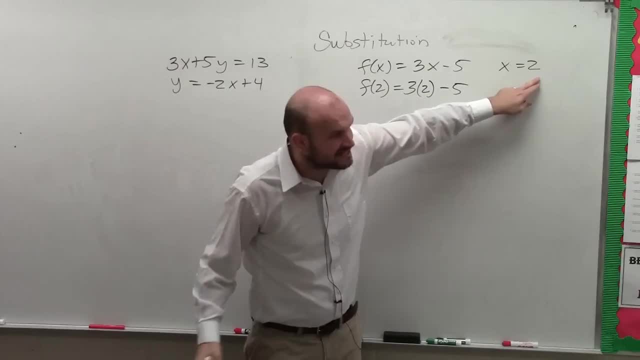 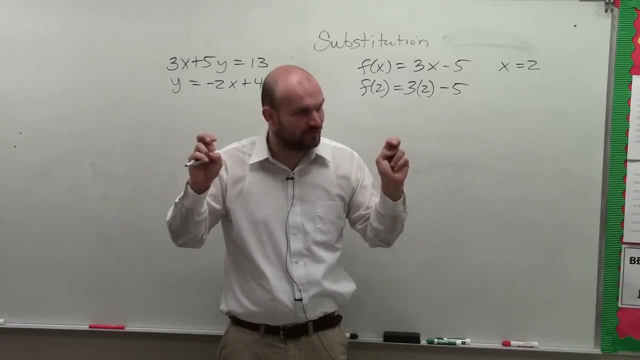 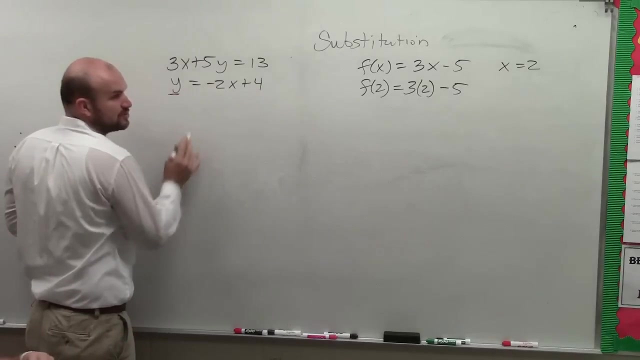 three times two minus five, because x was equal to two, Two was equal to x. You could replace them or substitute one for the other, correct? Now we're doing something very, very similar. Now y is not equal to a number, but it's equal to an expression. But we can still substitute. 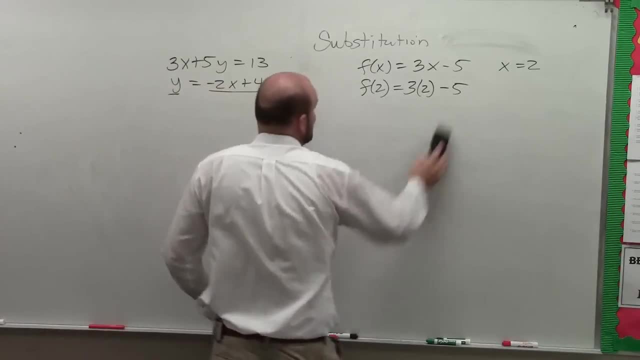 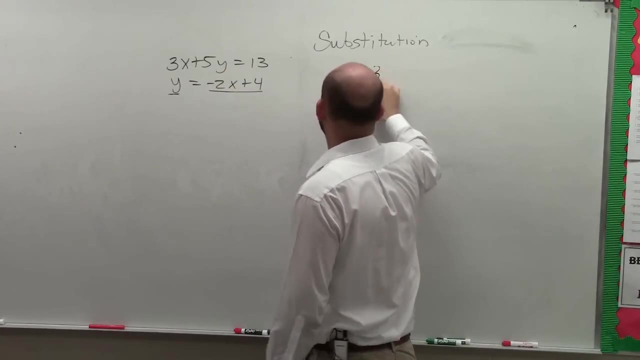 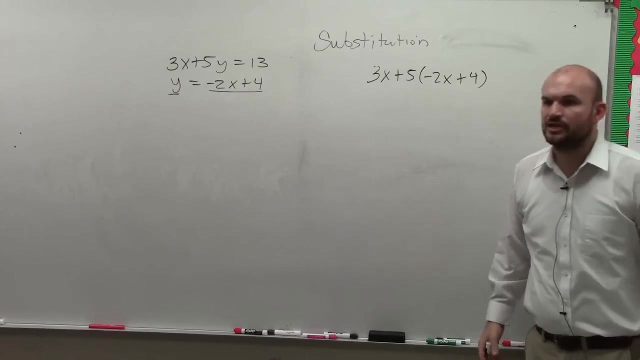 in that expression in for the variable. So that's exactly what I'm going to do. I'm going to substitute in my expression in for y into the other equation. So I have three x plus five times negative, two x plus four. Okay, Jade, Got it, You doing, alright. Okay, So, 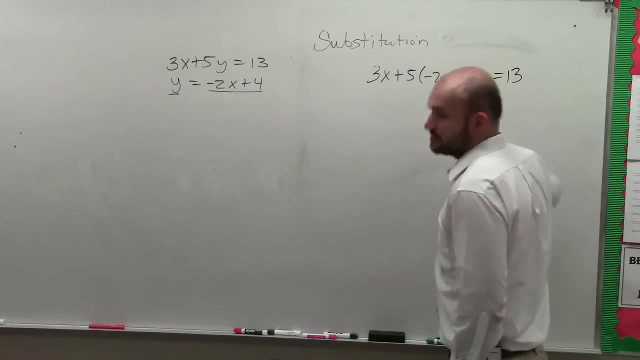 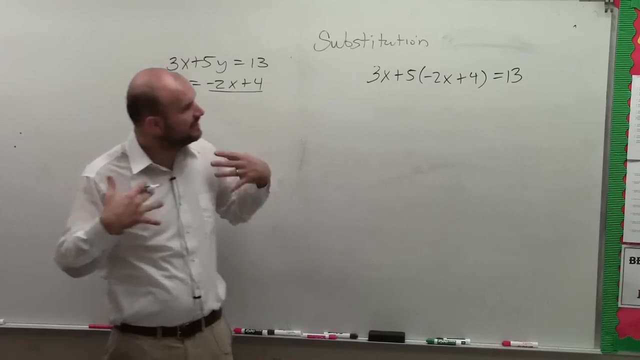 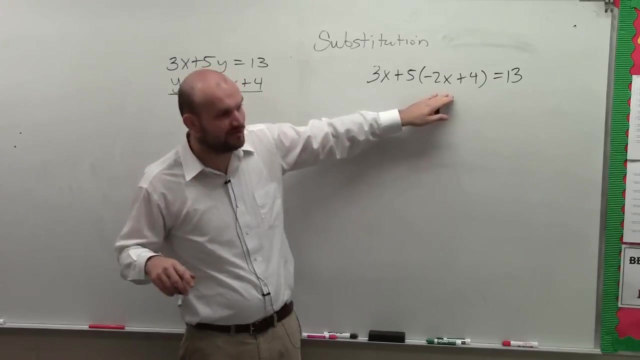 does everybody see? Does everybody see what I did? This is the big step, right there Now. the reason why that's so important is because now I have created an equation that only has one variable: x. Yes, it has two of them, but I'm only dealing with x. I'm not dealing. 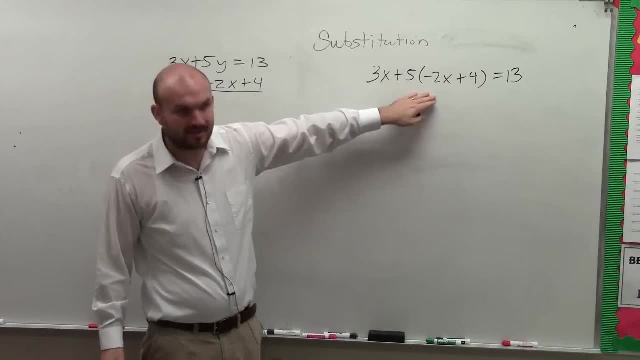 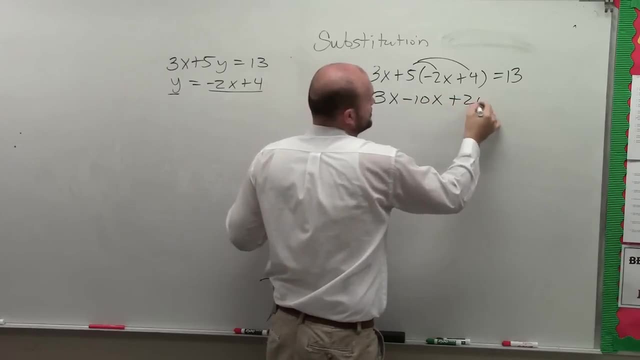 with x and y's. So now I can solve this. This is a multi-step equation. I can solve this, So I apply a distributive property. So I have three x minus ten x plus five times negative. seven x plus twenty equals thirteen. Three x minus ten x is negative. seven x plus twenty. 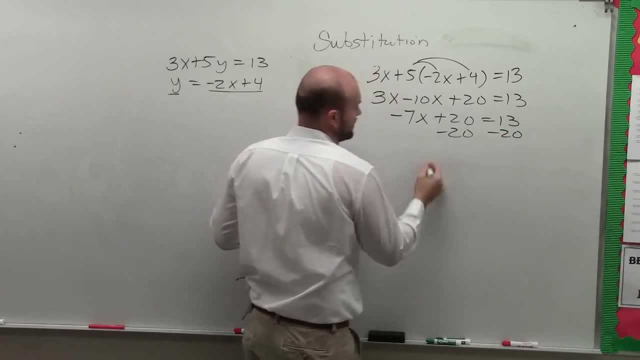 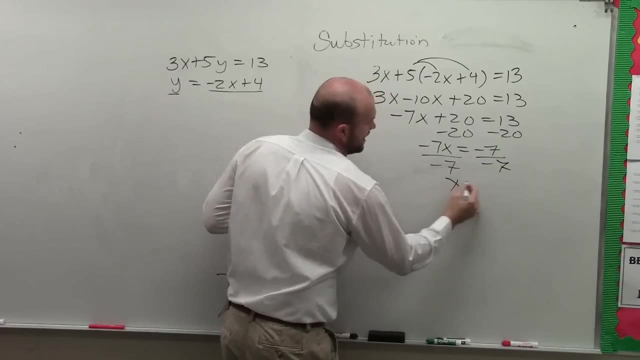 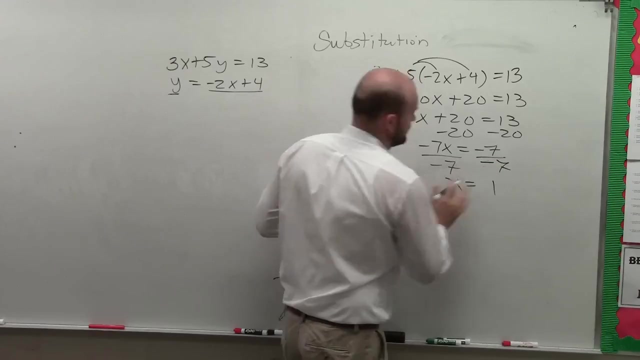 equals thirteen Subtract twenty. Subtract twenty. Negative seven: x equals negative seven Divide by negative seven. Divide by negative seven: X equals negative one, Positive one, Thank you. Negative seven divided by negative seven is positive one. So does everybody see. 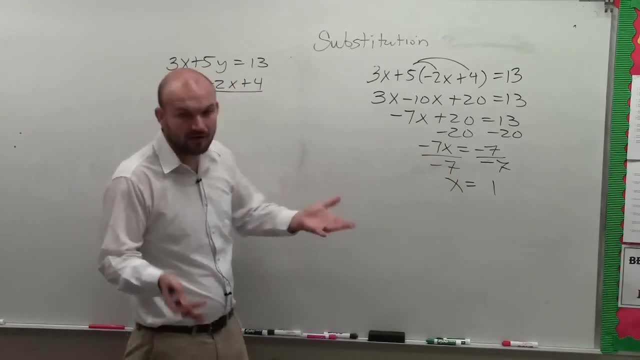 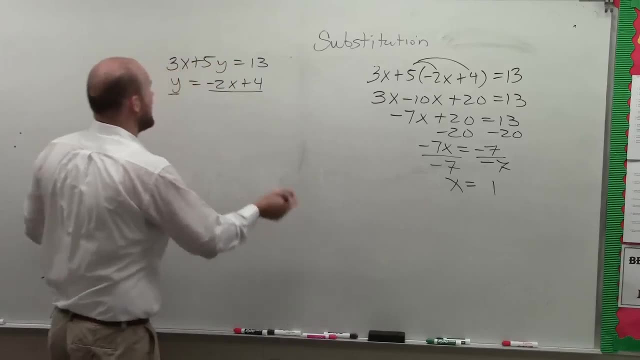 that Now I know the value of x. But again, when we're solving, remember when we did the intersection- we had an x and y coordinate where they intersected right. So we had x was equal to y. So now I'm going. 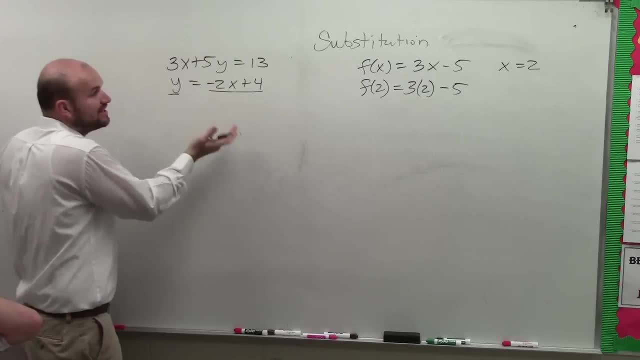 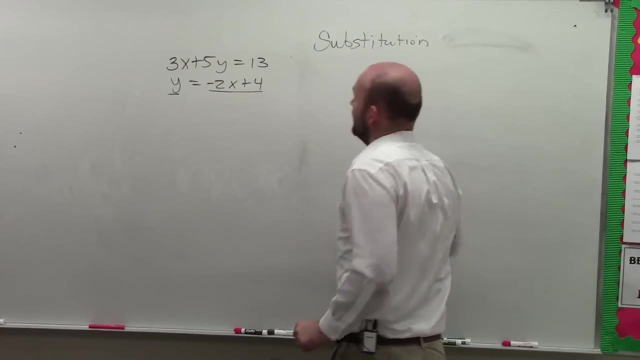 equal to a number, but it's equal to an expression. But we can still substitute in that expression in for the variable. So that's exactly what I'm going to do: I'm going to substitute in my expression in for y into the other equation, So I have 3x plus. 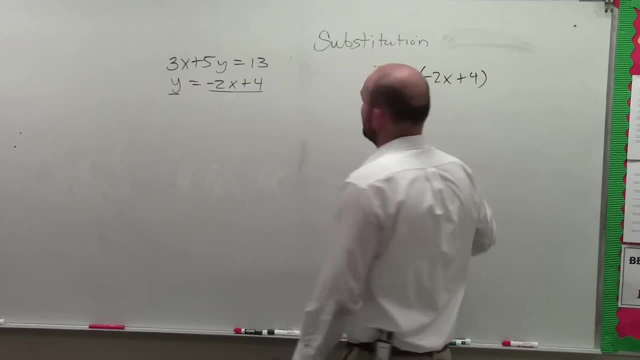 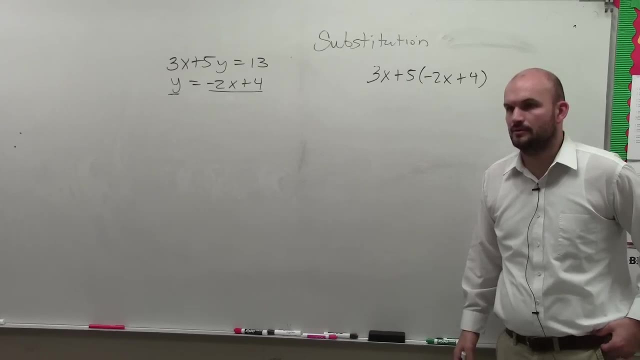 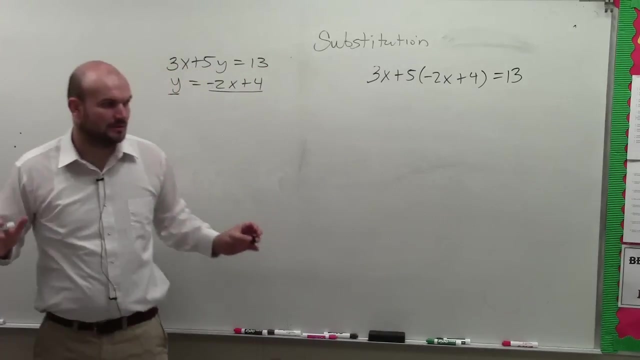 5 times negative: 2x plus 4.. Okay, Jade, Got it. You doing, all right, You okay. Okay, Does everybody see? Does everybody see? Let's see what I did. This is the big step right there Now. the reason why that's so important is: 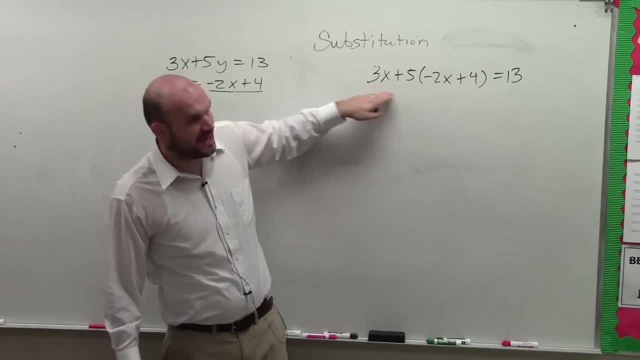 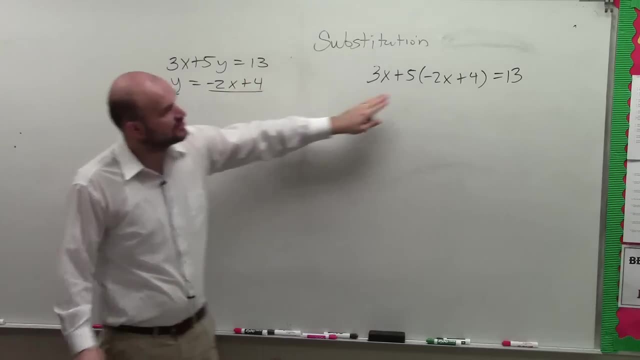 because now I have created an equation that only has one variable, x. Yes, it has two of them, but I'm only dealing with x. I'm not dealing with x and y's, So now I can solve this. This is a. 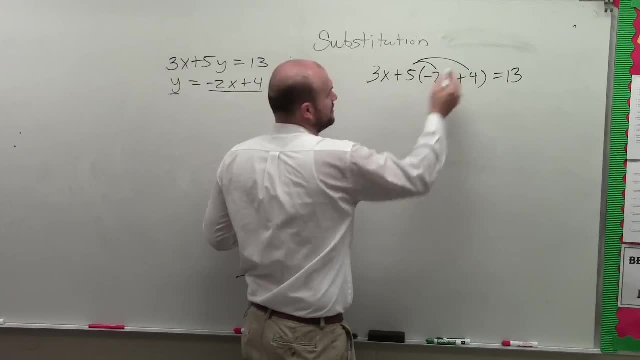 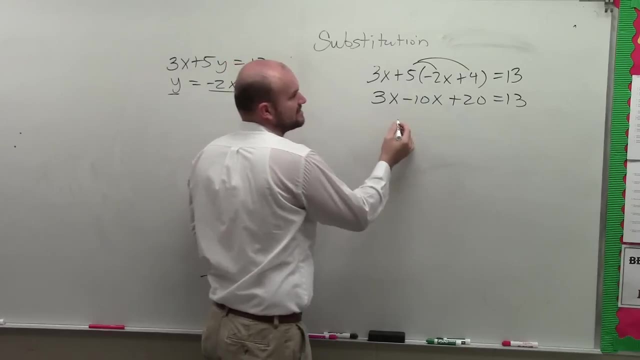 multi-step equation. I can solve this. So I apply distributive property. So I have 3x minus 10x plus 20 equals 13.. 3x minus 10x is negative. So I have 3x minus 10x plus 20 equals 13.. 3x minus 10x is: 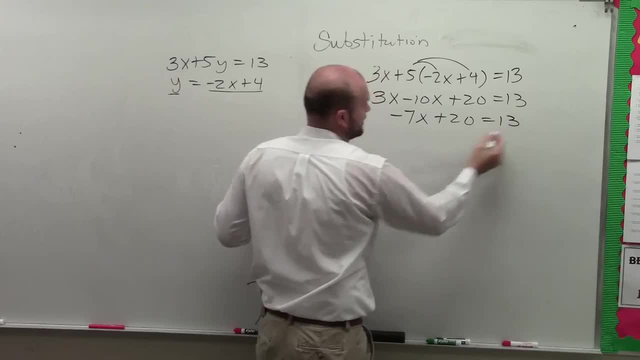 negative. So I have 3x minus 10x plus 20, equals 13.. 3x minus 10x is negative. So I have: 3x minus 10x is negative. So I have 3x minus 10x plus 20, equals 13.. Subtract 20, subtract 20.. Negative: 7x equals. 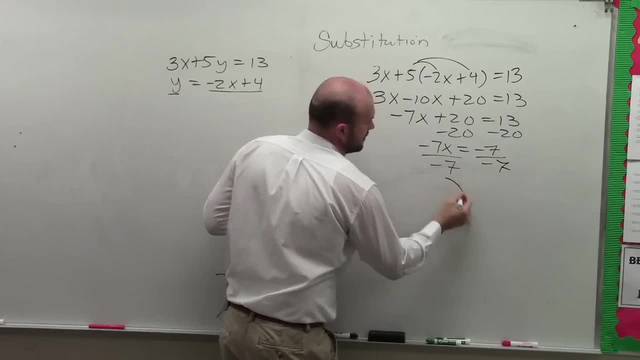 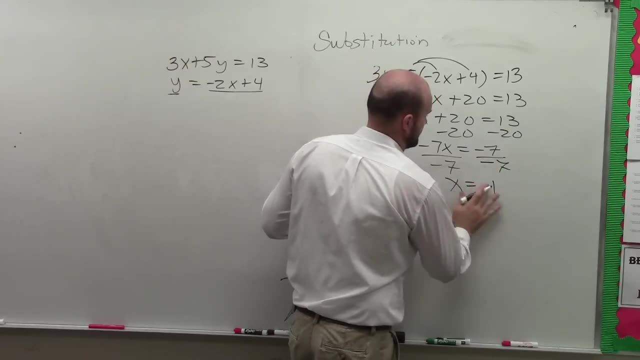 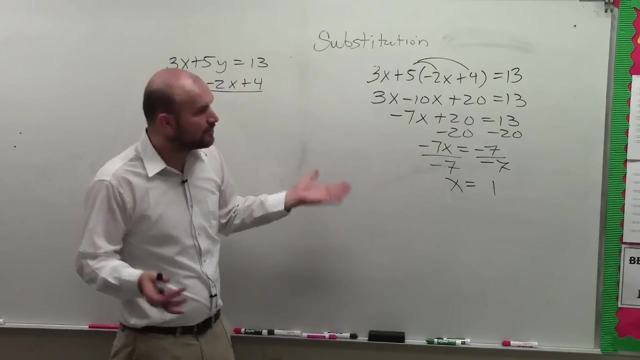 negative 7.. Divide by negative: 7. X equals negative 1. Positive 1.. Thank you. Negative 7 divided by negative: 7 is positive 1.. So does everybody see that? Now I know the value of x. But again, when? 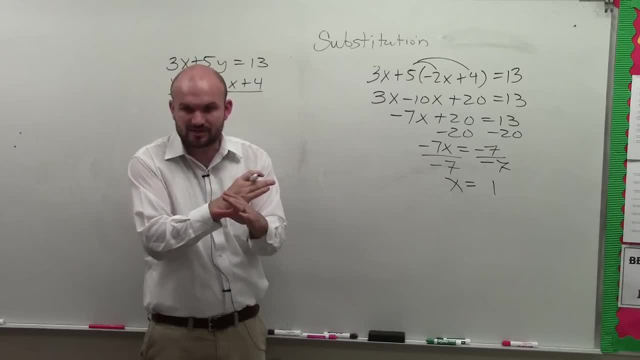 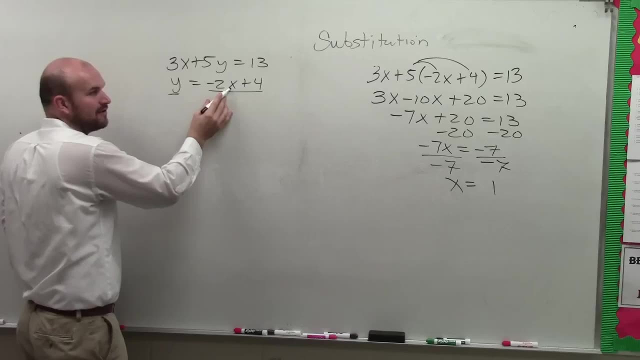 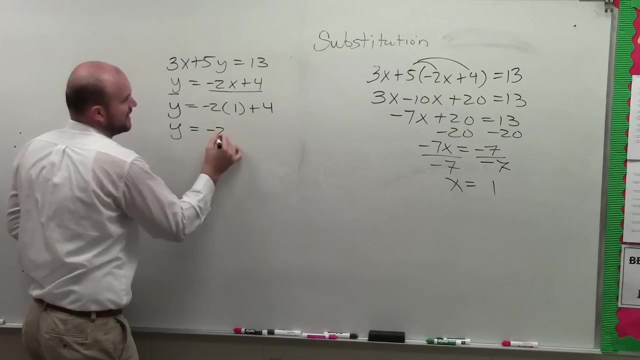 we're solving. remember when we did the intersection, we had x and y where they intersected right. So we had x was equal to y. So now I'm going to take my value of x and plug it in for x. So I have y equals negative 2 times 1 plus 4.. So y equals negative 2 plus 4.. 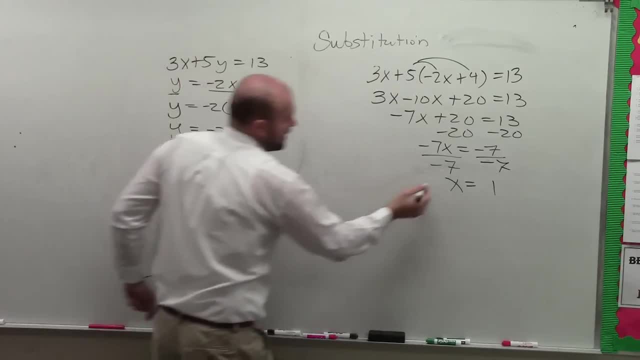 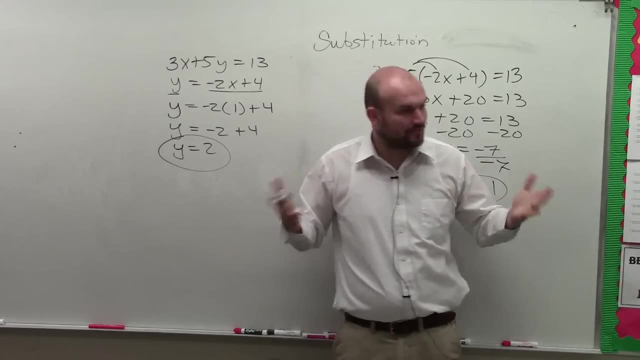 y is equal to 2.. So now I know the value of y and I know the value of x. Now, on an equation, if you were to think about this graphically, if we know the x and the y coordinate, that represents where they intersect, right. So then, what kind of solution? Is this? consistent or inconsistent?